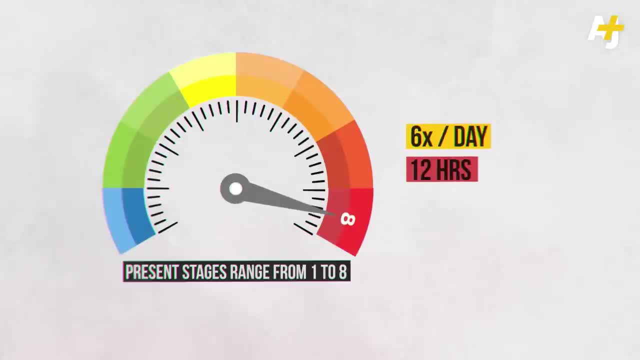 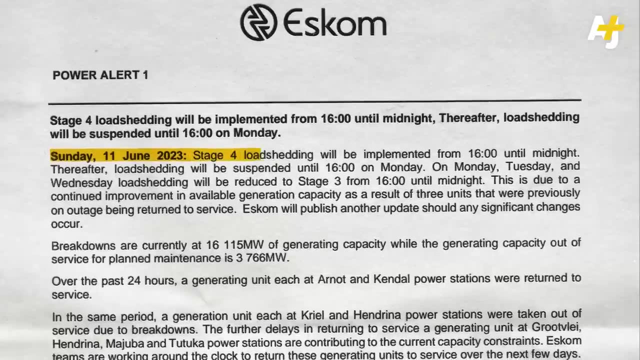 Stage eight is worse. Load shedding would occur six times a day or for 12 hours, depending on the schedule. On June 11th, ESCOM issued this power alert. Stage four load shedding will be implemented from 1,600 hours until midnight. 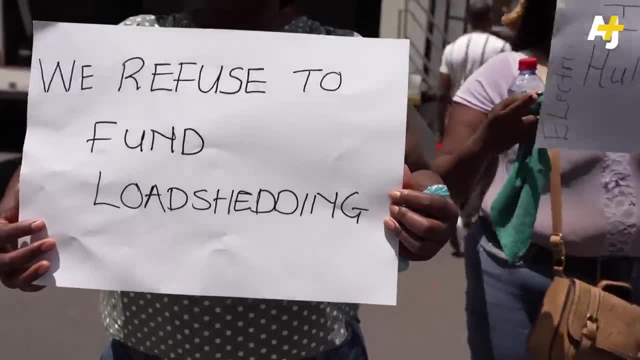 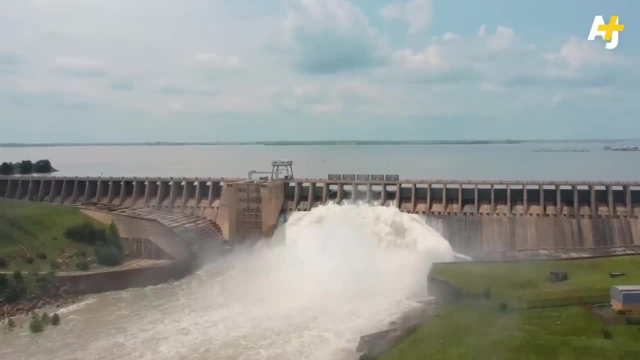 Can you imagine being without power regularly for eight hours? Well, South Africans have been dealing with blackouts like this since 2007.. These blackouts rattle every aspect of daily life, affecting hospitals, education and the environment. These blackouts rattle every aspect of daily life, affecting hospitals, education and the environment. 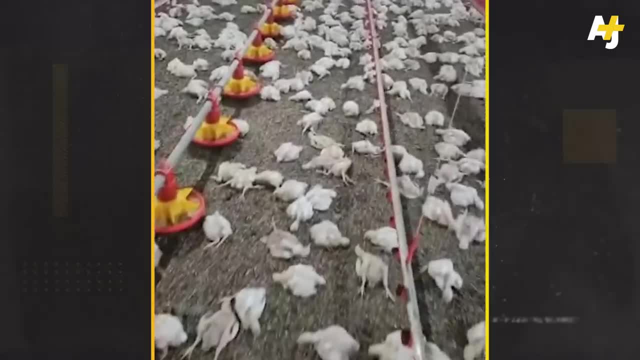 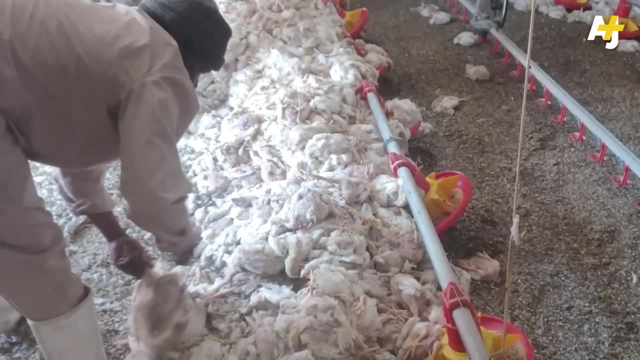 These blackouts rattle every aspect of daily life, affecting hospitals, education and the environment And the food and water supplies. You might remember this viral video of workers removing 50,000 dead chickens from a farm. The birds reportedly suffocated when power outages caused the ventilation system to stop. 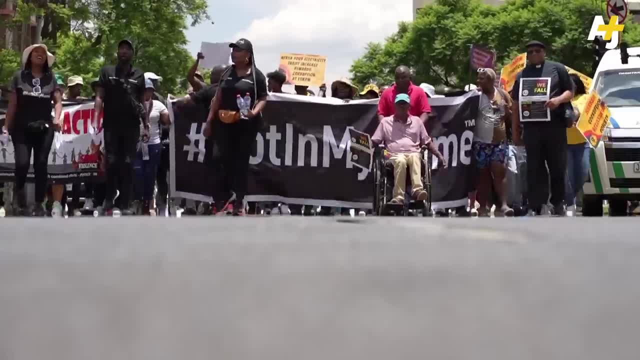 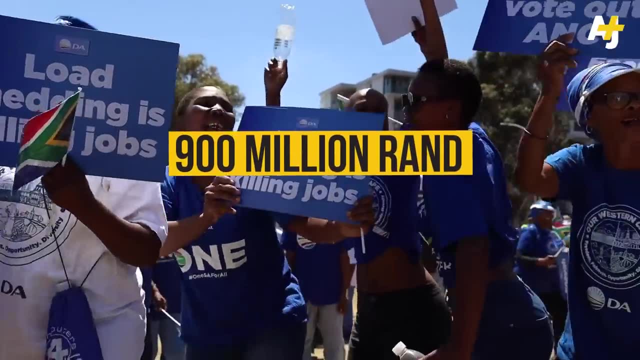 Then there's South Africa's economy. Load shedding is both creating and adding to the nation's high unemployment rate and its faltering economy, Costing South Africa almost 900 million rand, or $48 million a day, Because load shedding is a rotational rationing. 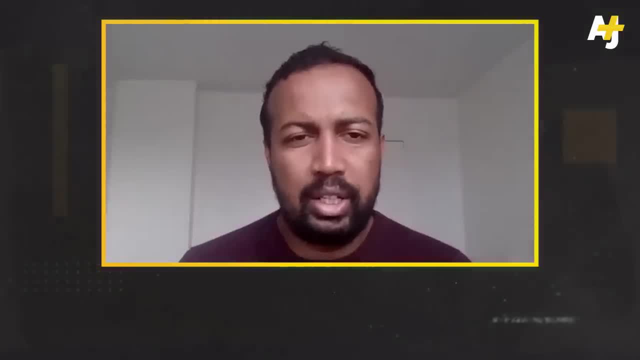 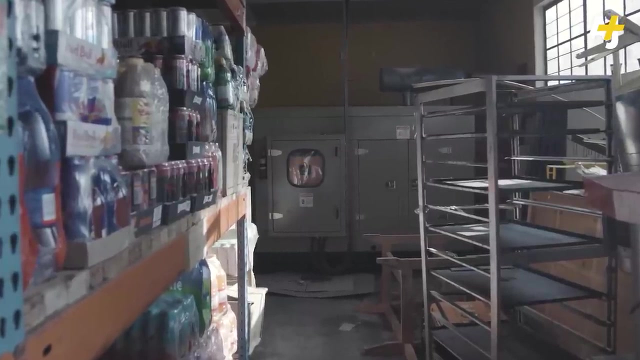 Everyone in South Africa is impacted by load shedding. Of course, different people and organizations are able to insulate themselves from the impact of load shedding because they have the resources- Resources like solar energy, battery systems and diesel generators- And those who don't have access are hit the hardest. 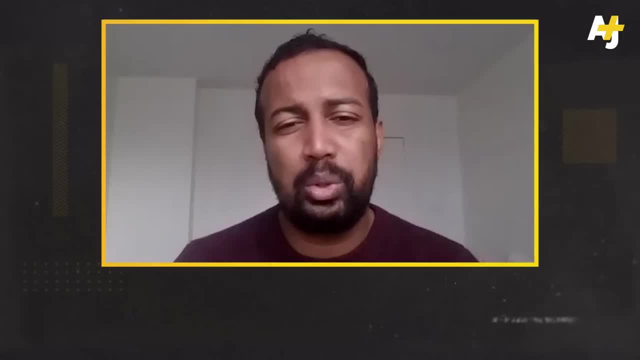 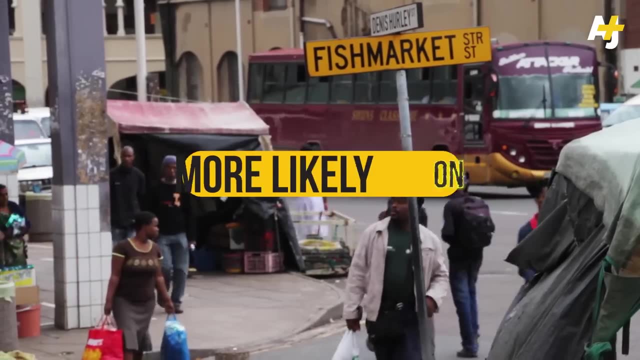 It's drifting people more into energy poverty. People are switching to fuels like paraffin and candle burning for lighting. Some Black communities are 3.5 times more likely to have power cuts than majority white areas. ESCOM has even been accused of using longer outages in Black neighborhoods. 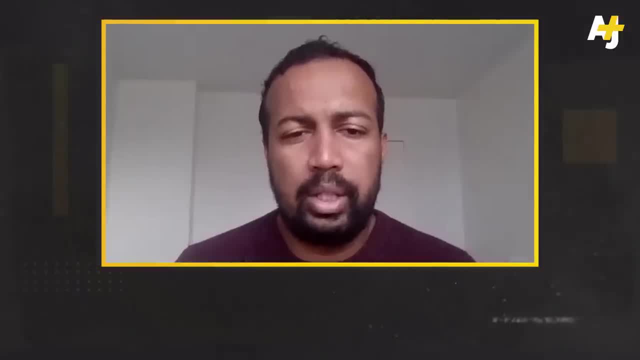 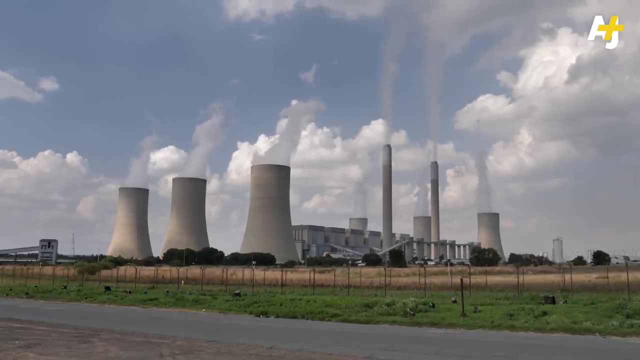 The particular hours that were being load shed for Black working class users, especially in townships, was very punitive, was at the precise times that they may be returning from home And it was observed to be racially biased. But energy racism is not new to South Africa. 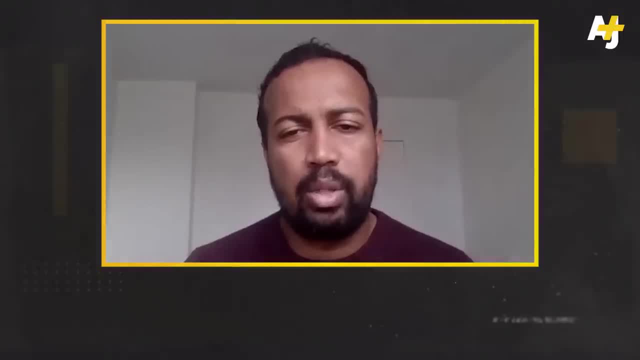 Part of the crisis that we are seeing is the lack of the ability of the ANC government to establish a new progressive economic paradigm in the post-apartheid era that can both industrialize but also can extend its benefits to the broader population, to the Black working class in particular. 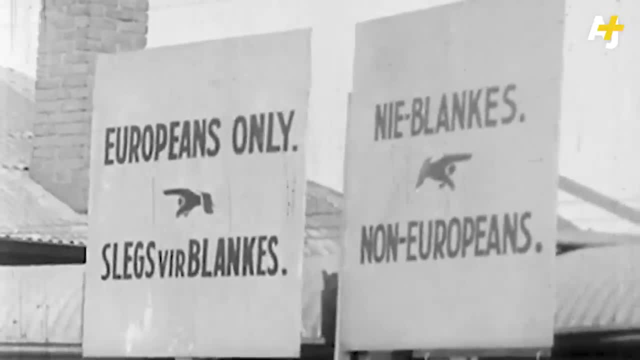 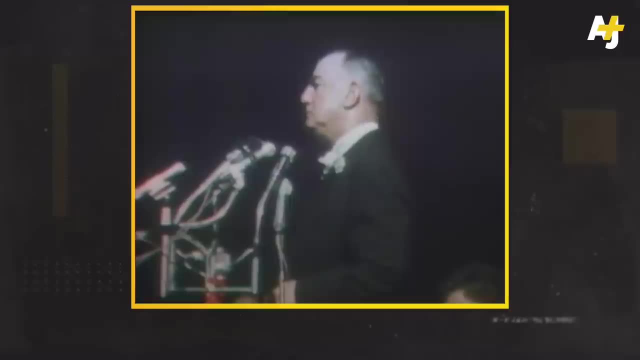 So let's take a step back. Apartheid was a legal system for racial segregation against non-white residents of South Africa. It began in 1948.. After the National Assembly of the United States of America, the National Party were voted into power by the white minority. 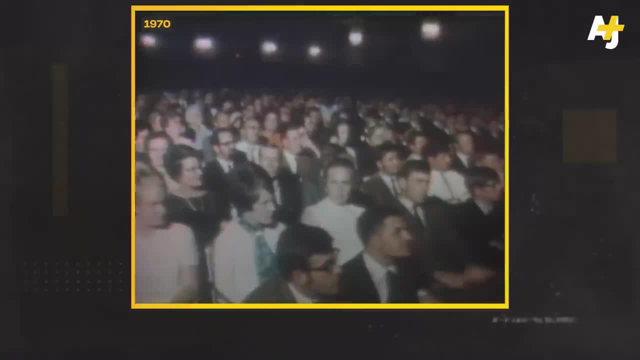 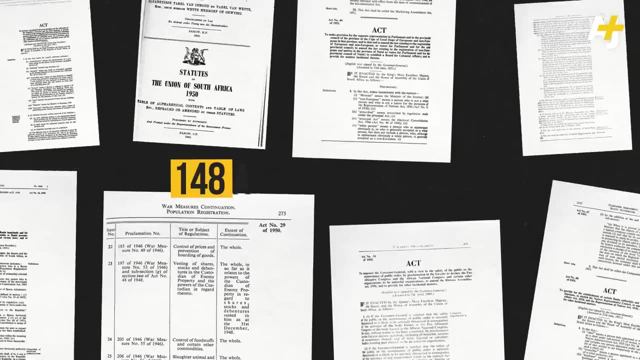 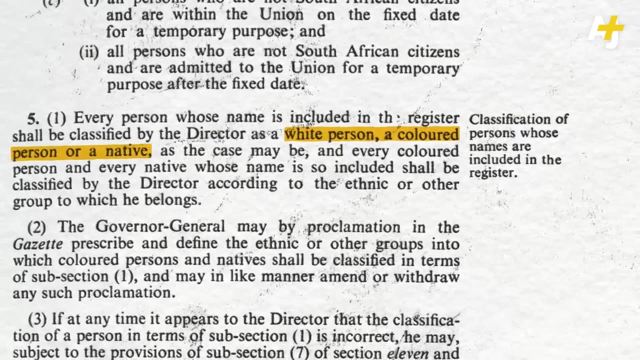 The party governed South Africa for decades. We have every right to maintain our identity as whites. From 1948 to 1971, the National Party instituted 148 apartheid laws dividing people by race: white colored, native or Black, and Asian or Indian. 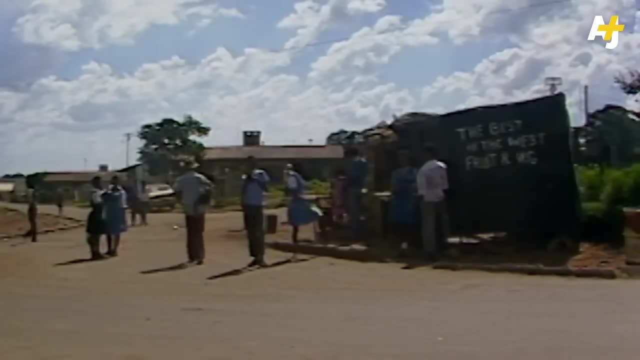 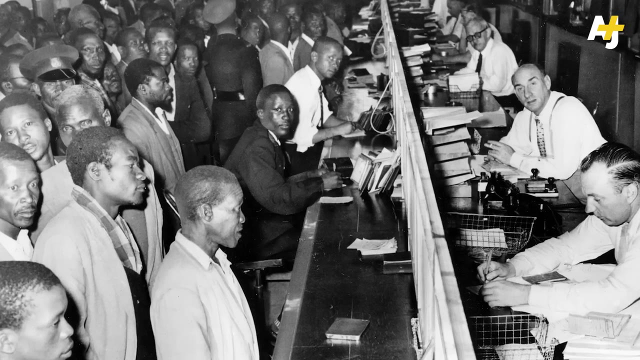 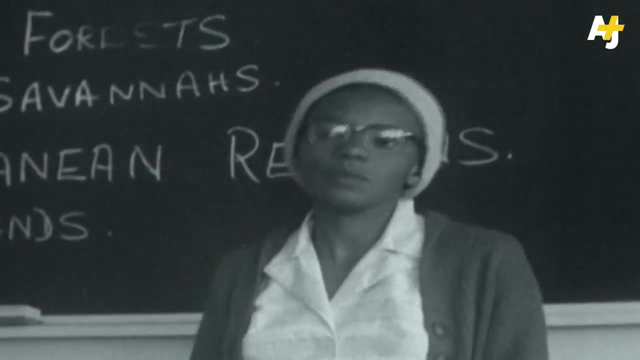 Race controlled every aspect of life in South Africa, from jobs, public facilities and transportation to education and health systems. Black people even had to carry passbooks which restricted where they could travel and stipulated where they worked. Under apartheid, 3.5 million non-white South Africans were also removed from cities and their homes. 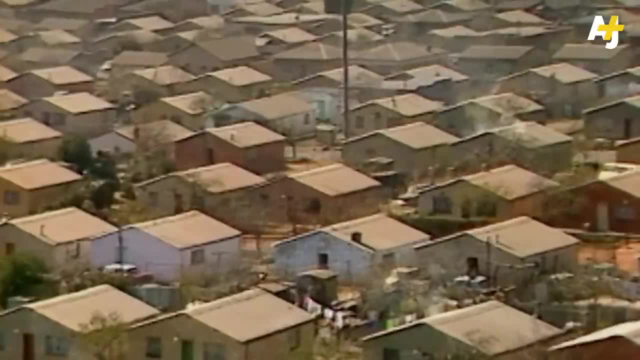 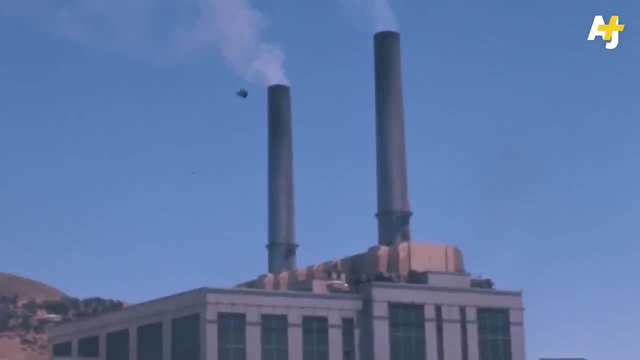 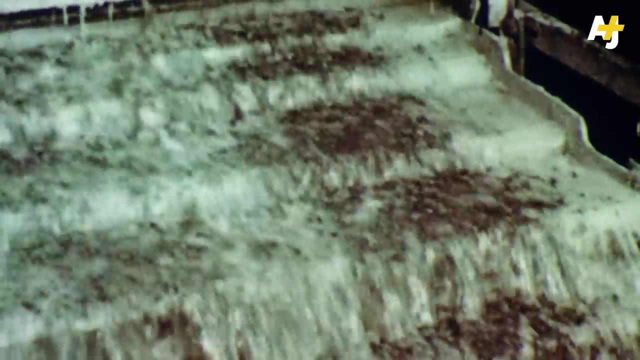 and relocated to segregated urban townships or mostly rural bantustans During this period. ESCOM was the electricity utility of the settler colonial apartheid state. It principally provided electricity to the country's ruling white minority and subsidized service for the country's manufacturing and mining. 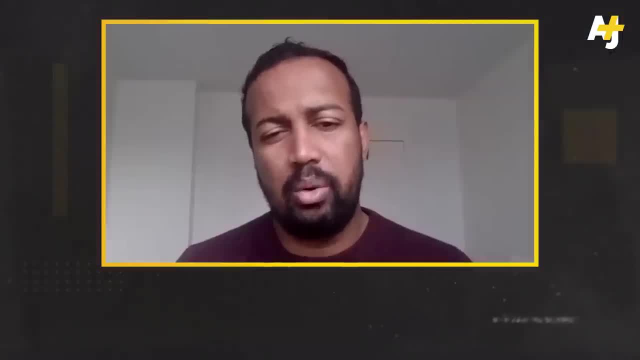 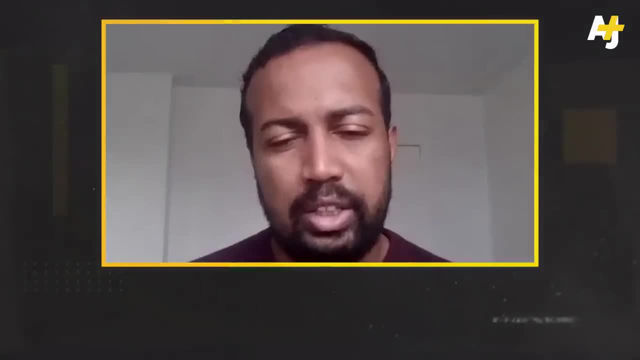 The electricity had been as integrated as it is now into what people consider to be the basic elements of living a decent life. So there's very low levels of rural electrification. The inequality of infrastructure was mapped onto the inequalities enshrined in the apartheid project. 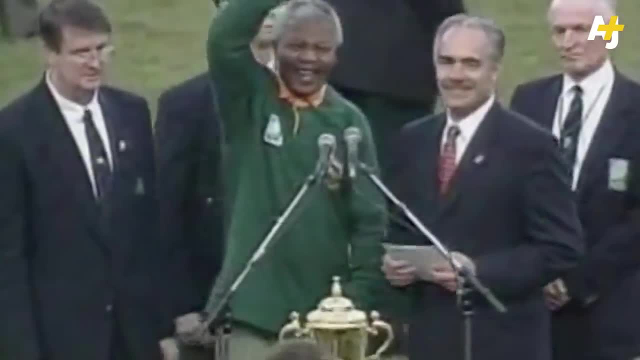 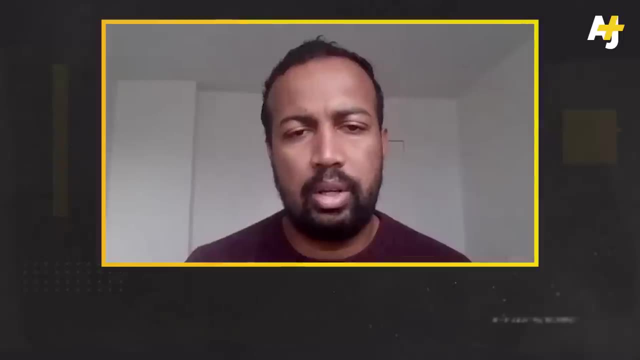 By 1994, apartheid had ended, but only about half of South Africans had electricity. Nearly all white households had access, but many Black families had none. It was at the turnover of the new government that ESCOM was impulsed to redistribute access to basic services. 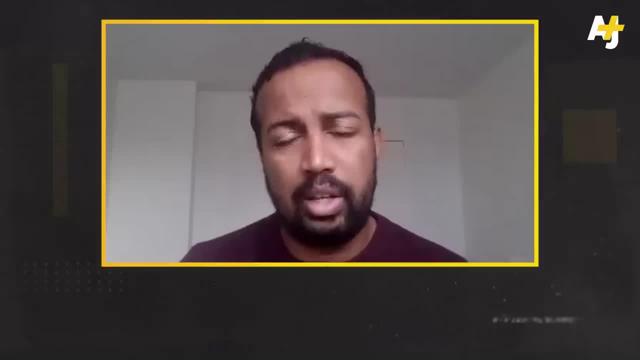 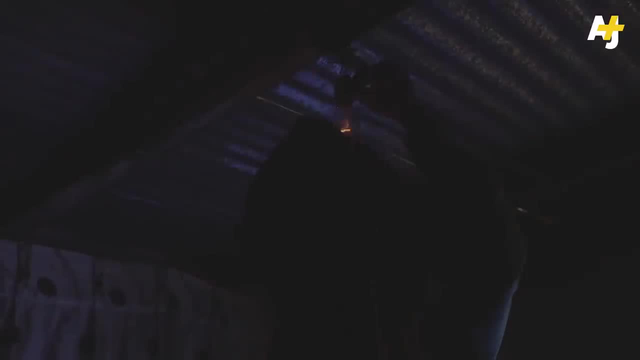 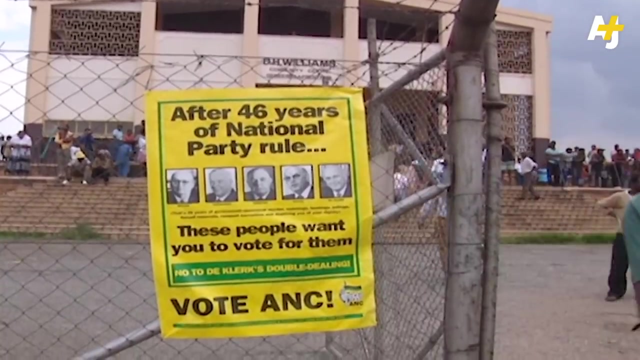 We had a mass rural electrification scheme that was largely financed through public funds. We had the concept of free basic services, of free basic electricity. South Africa's new ANC government came to power promising to serve the country's poor, but its leaders soon embraced pro-business, neoliberal policies that worsened inequality. 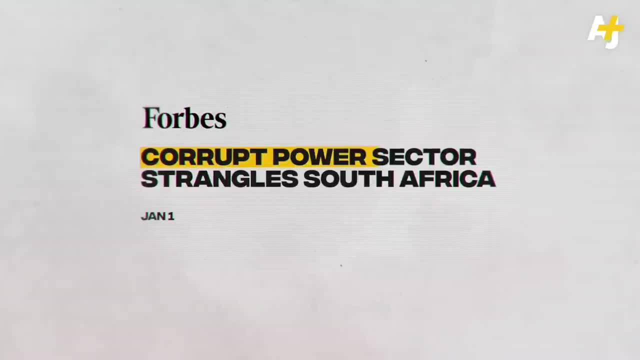 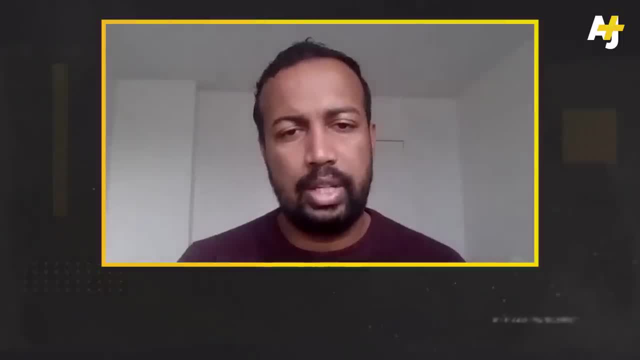 and many of its members were forced to leave the country and many of its members were forced to leave the country. Inadequate planning was done to ensure that there is sufficient generation capacity procured, So we failed to plan, but also we failed to maintain where we have leads to poor performance. 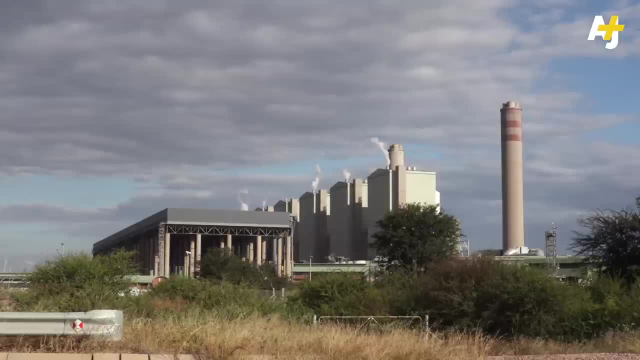 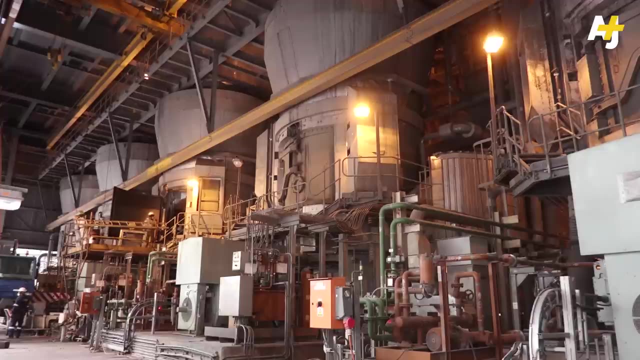 In 2007,, South Africa started construction on two of the world's largest coal-fired plants: Wadupi and Kesele. They were touted as the answer to load-shedding and the country's energy crisis, But, due to design flaws and equipment failures, 16 years later. 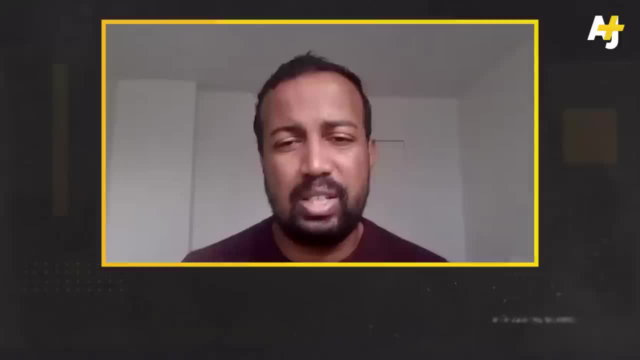 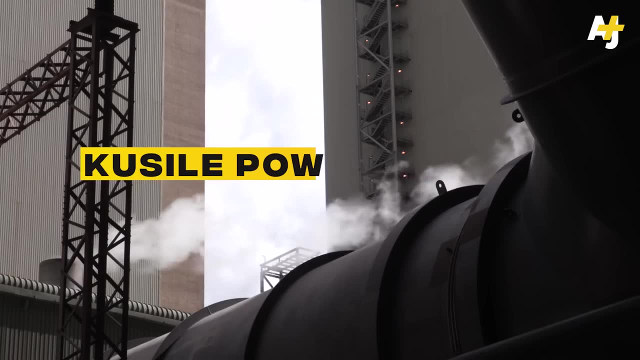 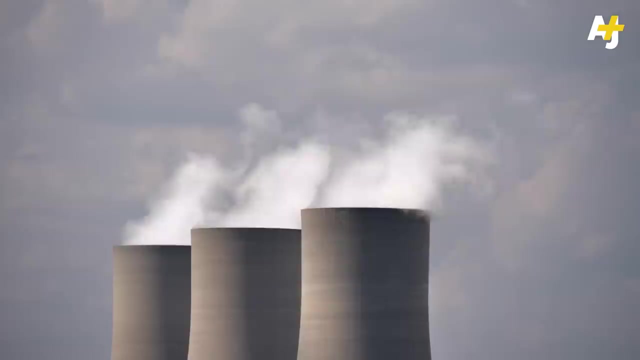 both the plants are operating well below 50% of their capacity. It's a devastating situation. Other estimates put one plant at 70% operational and the other at just over 37%. Currently, the South African government is focused on improving the performance of its existing coal fleet. 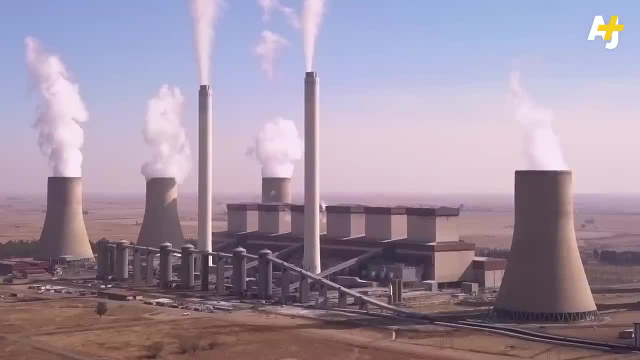 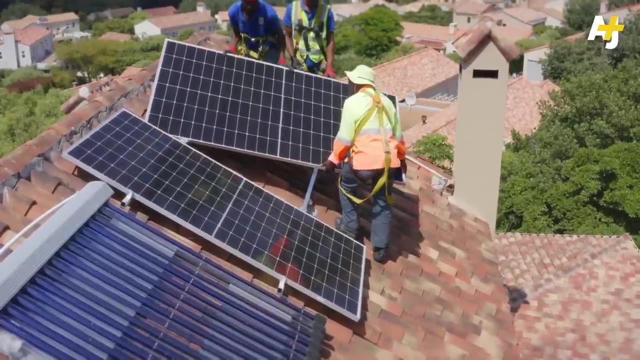 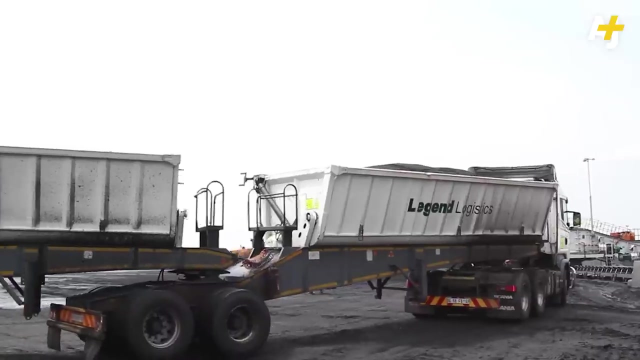 and procuring renewable energy from other producers. Regarding long-term solutions, there are calls for the country to cut its carbon emissions by transitioning to renewable energies like wind and solar. Ending reliance on fossil fuels and shifting to renewable energy is generally considered to be one of the most effective ways of fighting the climate crisis. 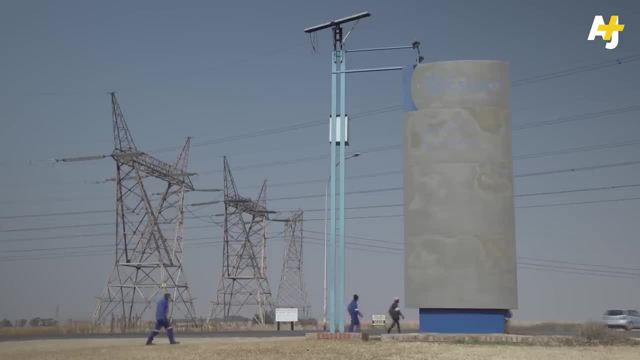 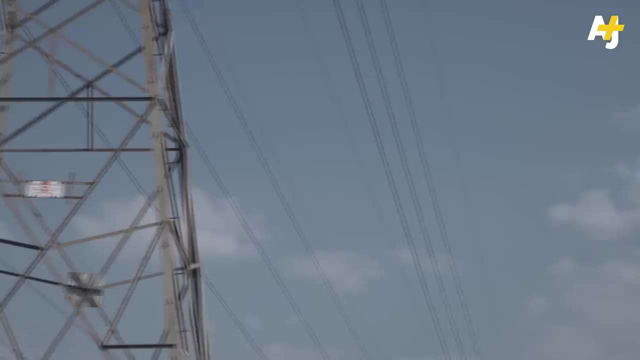 But it does come with challenges. First, South Africa's coal mines employ 90,000 people, And renewable energy is still often expensive, so many people can't afford to install systems that support it. Plus, South Africa's electricity infrastructure doesn't really support renewable energy. We are having issues implementing our capacity requirements And a lot of that has to do with transmission. So the transmission network, which is essentially the highways of the electricity system that is built throughout the country, it was never designed to accommodate a massive build-out. 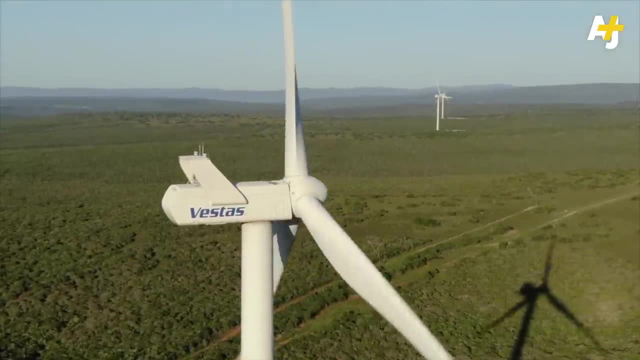 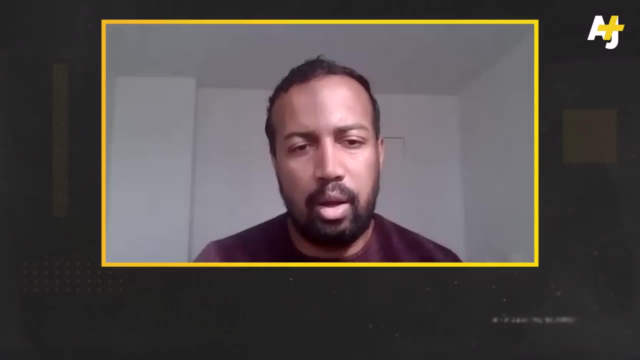 of renewable energy. But Kamanzi also warns that the transition to renewable energy in South Africa has become associated with privatization. Not all that glitters is gold. There are glittery plans that are being made in international forums to say South Africa is going green. 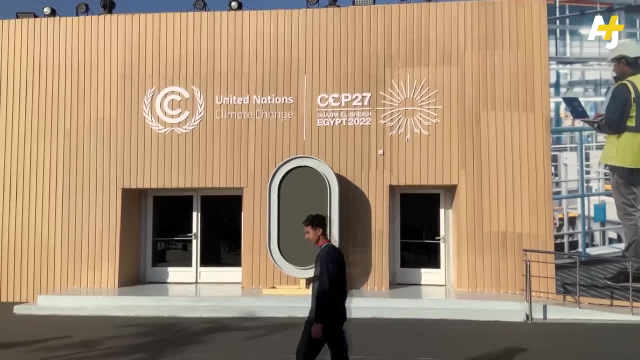 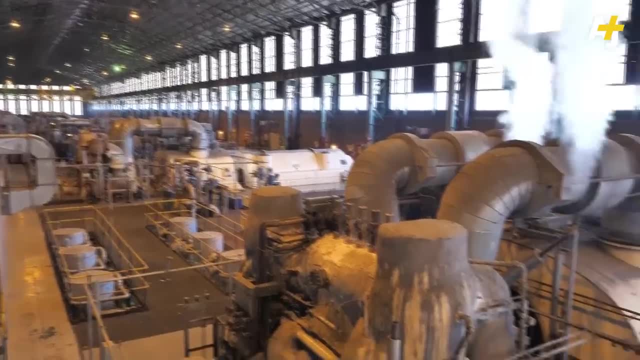 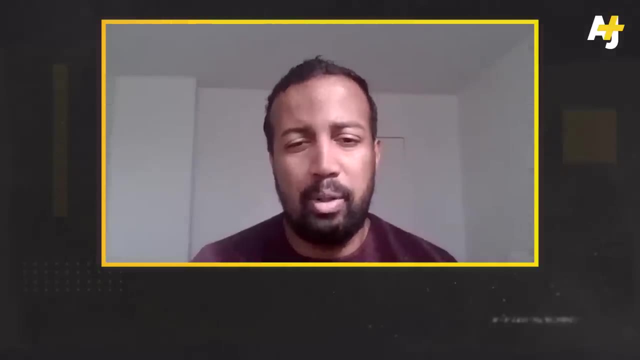 And that there will be all these jobs created, But that's not necessarily true. Shortly after South Africa announced plans to go green at the COP27 summit, the coal-fired Kamanzi power station was shut down, Which, without the requisite planning that have left many people in the plant and people. 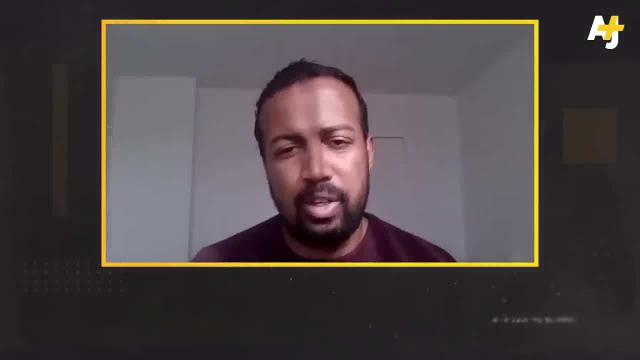 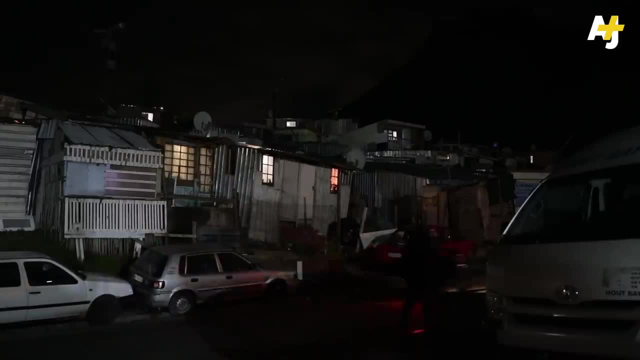 indirectly employed in the area, you know, without livelihood. Other countries dealing with load shutting are also trying to figure out how to solve this growing problem, How South Africa moves to make an equitable world. And if that's not the case, how can we make a sustainable transition to renewable energy?